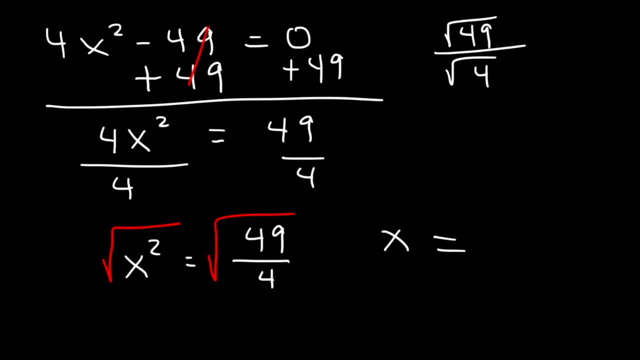 So what is the answer? What is the square root of 49 over 4?? If you need to find the square root of a fraction, this is equivalent to square root 49 over square root 49.. root: 4.. You want to take the square root of each number separately? The square root of 49 is 7.. 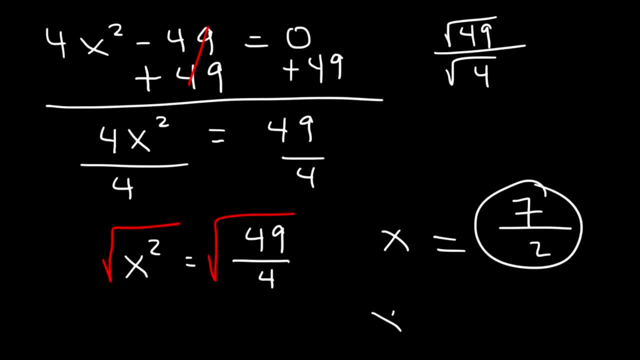 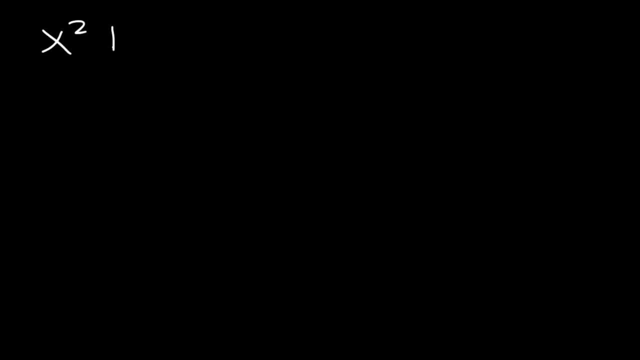 The square root of 4 is 2.. So the answer is positive, 7 over 2, and also negative, 7 over 2.. Now what about this? one x squared plus 4 is equal to 0.. First we need to subtract 4 from both sides, So x squared is equal to negative 4.. 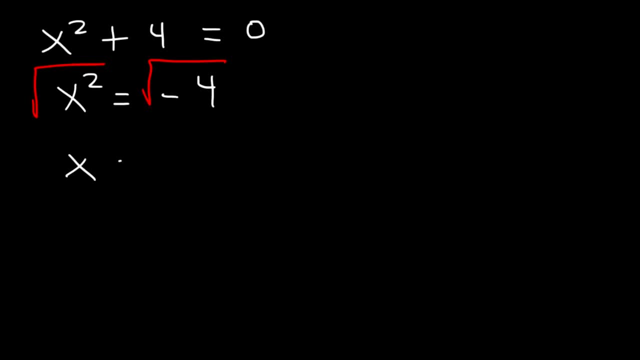 Now, what is the square root of a negative number? The square root of a negative number is not a real number, So we're going to get an imaginary solution. I'm going to write this as the square root of 4 times the square root of negative 1.. 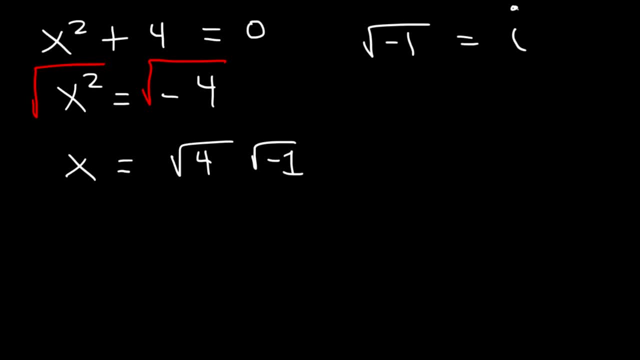 You need to know that the square root of negative 1 is i. This is going to be plus or minus. The square root of 4 is 2.. So the final answer is plus or minus 2i. Positive 2i. 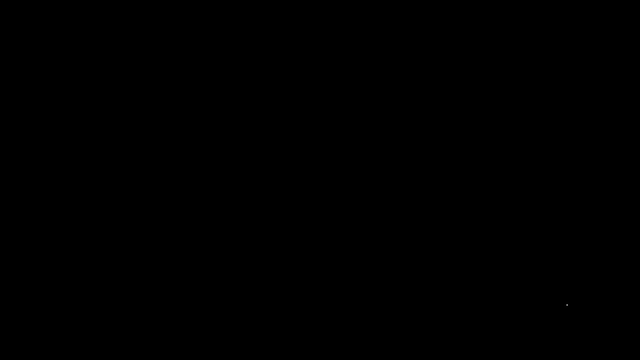 And negative 2i. Try this one. Let's say that x minus 5 squared is equal to 9.. Find the value of x. The first thing we should do is take the square root of both sides, The square root of x minus 5 squared. the twos will cancel. 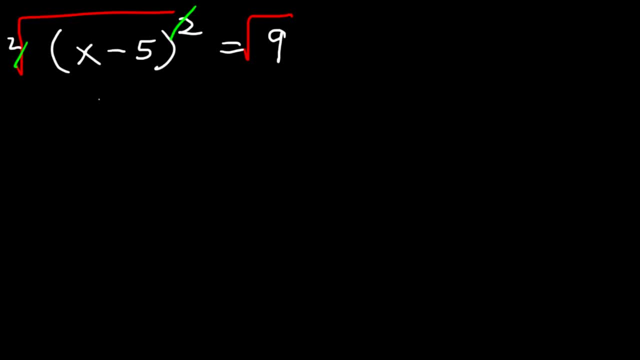 The square and the square root will disappear. So on the left side all we have is x minus 5.. And the square root of 9 is equal to 2 things Plus or minus 3. So x minus 5 is equal to positive 3.. 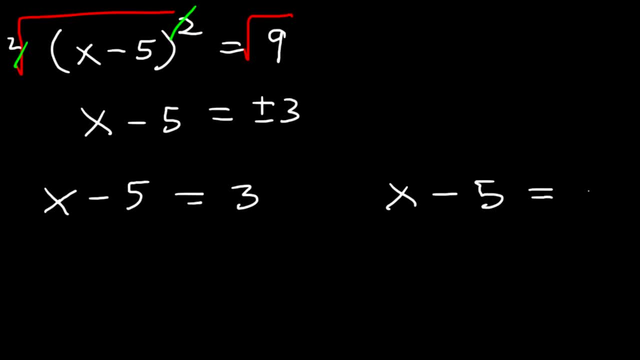 And also: x minus 5 is equal to negative 3.. Here let's add 5 to both sides, So 3 plus 5 is 8.. So this is one of the answers: x is equal to 8.. Now if we add 5 to negative 3,, 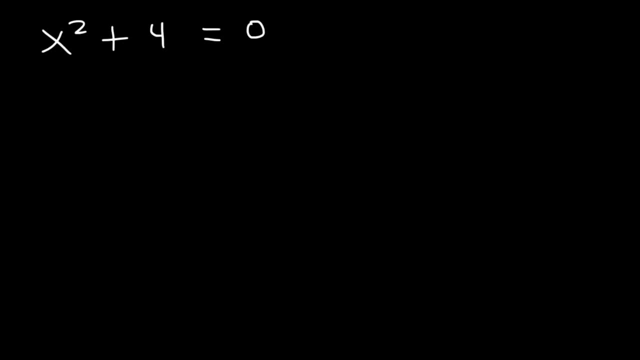 Now what about this one? x squared plus 4 is equal to 0.. First we need to subtract 4 from both sides, So x squared is equal to negative 4.. Now what is the square root of a negative number? The square root of a negative number is not a real number. 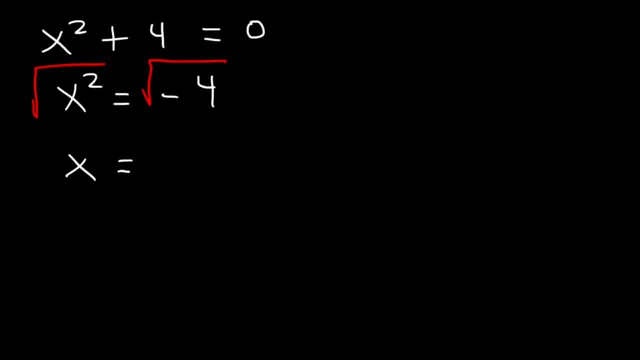 So we're going to get an imaginary solution. I'm going to write this as the square root of 4 times the square root of negative 1.. You need to know that the square root of negative 1 is i. This is going to be plus or minus. The square root of 4 is 2.. 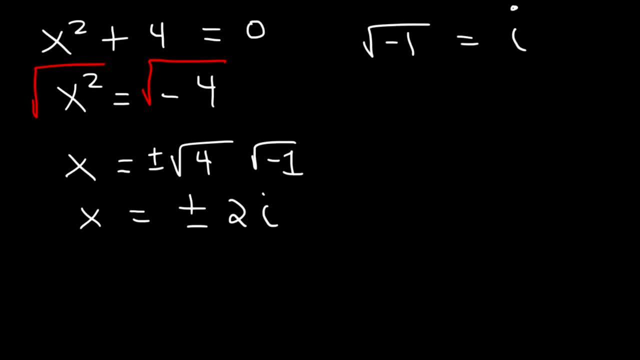 So the final answer is plus or minus 2i, Positive 2i And negative 2i. Try this one. Let's say that x minus 5 squared is equal to 9.. Find the value of x. The first thing we should do is take the square root of both sides. 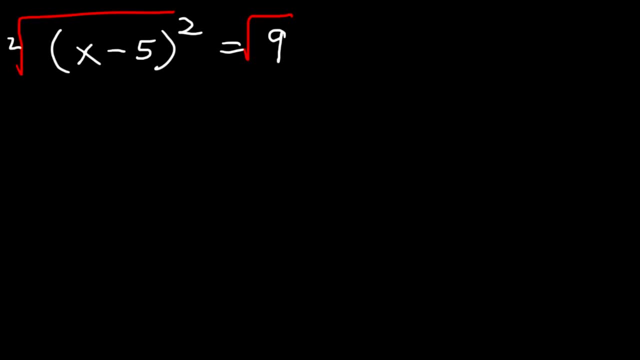 The square root of x minus 5. squared, the twos will cancel The square and the square root will disappear. So on the left side all we have is x minus 5.. And the square root of 9 is equal to 2 things plus or minus 3.. 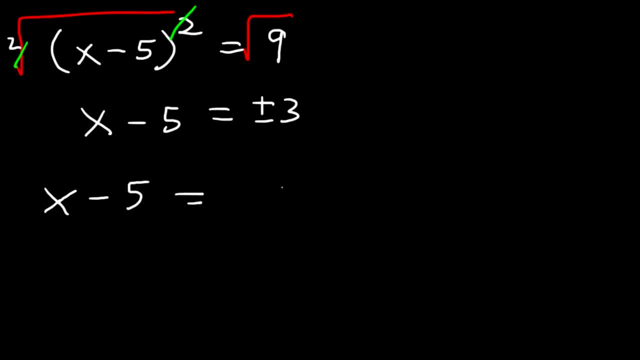 So x minus 5 is equal to positive 3. And also x minus 5 is equal to negative 3. Here let's add 5 to both sides, So 3 plus 5 is 8.. So this is one of the answers: x is equal to 8.. 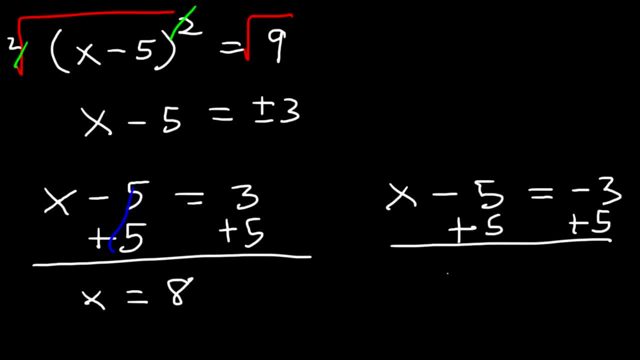 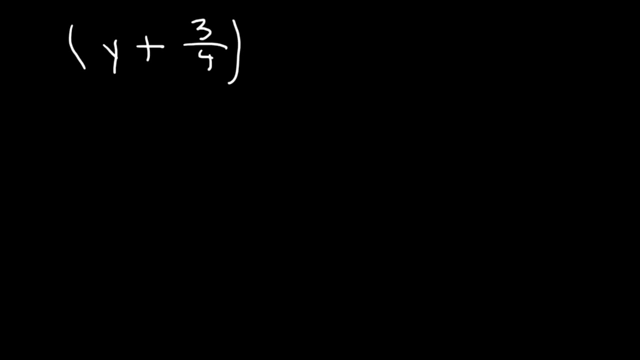 Now, if we add 5 to negative 3, that will change the answer, will give us positive 2.. So x is equal to 8 and it's equal to 2 as well. So we have two answers. Let's try another one, like that: y plus 3 over 4 squared is equal to. 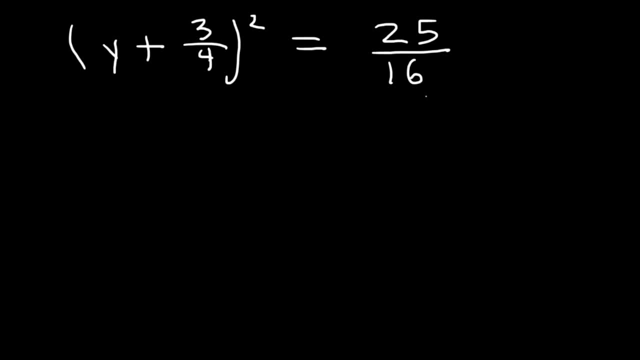 25 divided by 16.. Feel free to pause the video and try this problem. So let's start by taking the square root of both sides. So on the left the square will disappear. It's just y plus 3 over 4.. On the right, the square root of 25 is 5, the